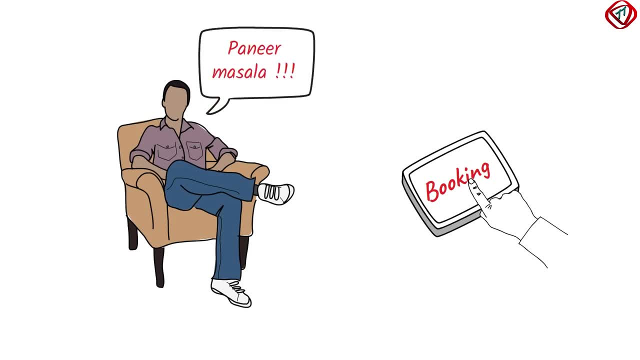 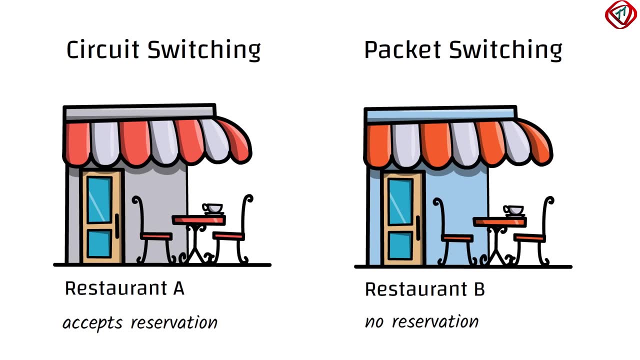 I can immediately be seated and can order my meal. On the other hand, restaurant B does not accept reservation, So when I arrive at the restaurant I may have to wait in queues before I can be seated. Circuit switching is analogous to restaurant. 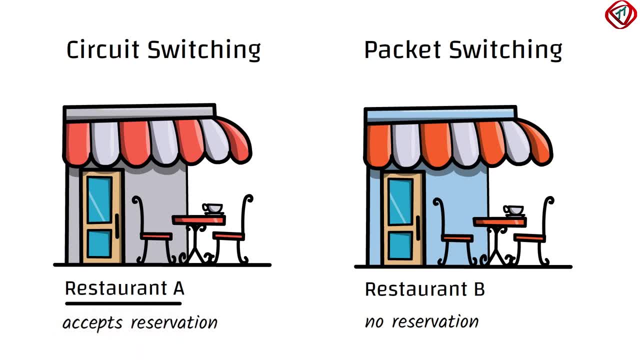 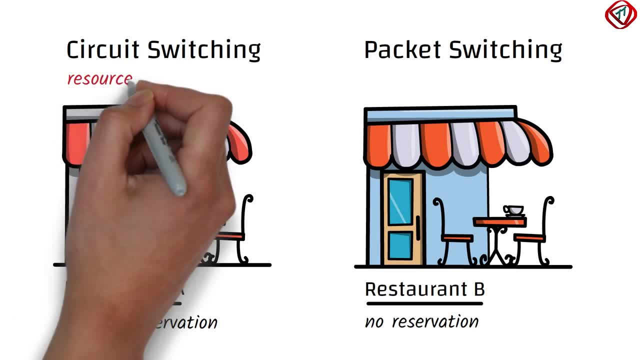 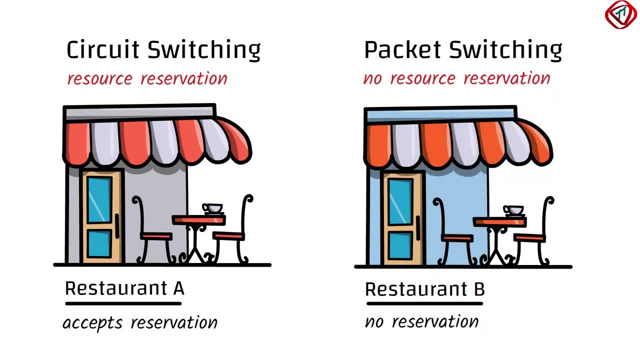 A, which accepts reservation. On the other hand, packet switching is analogous to restaurant B, which does not accept the reservation. That is, in circuit switching. resources are reserved for the communication session. On the other hand, resources are not reserved in packet switching. Having packet switching already discussed, 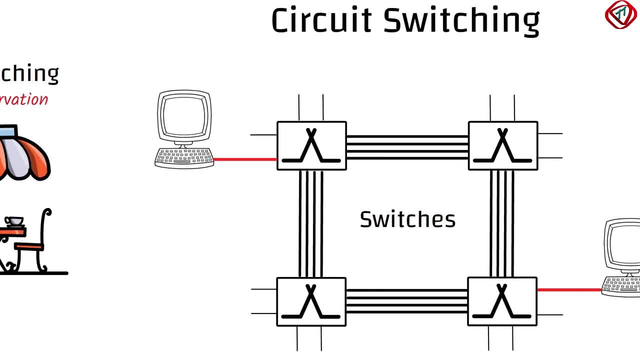 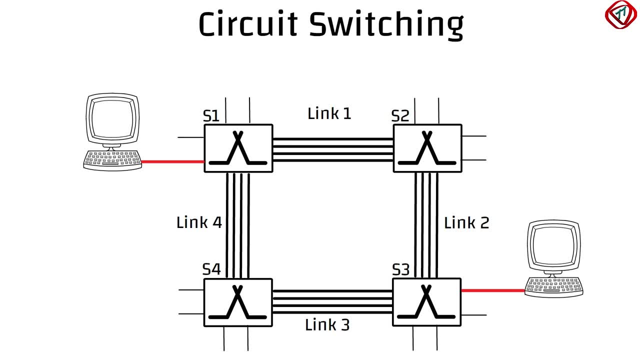 in earlier video. let us focus on circuit switching. Consider a network containing 4 switches interlinked by 4 links. Each link has four connections or channels. Host A and Host B are directly connected to the switches. If host A wants to communicate host B, the network first. 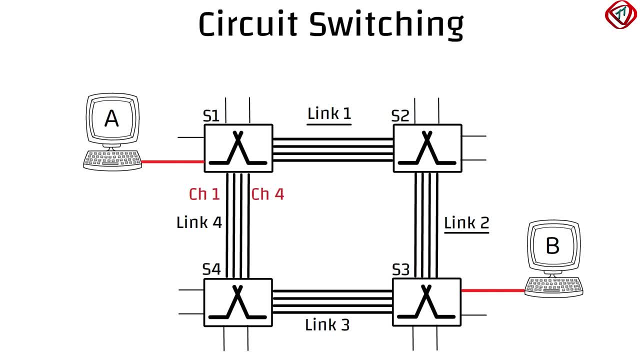 deserves a channel in the first and second link, say channel 1 in link 1 and channel 2 in link 2.. The combination of channels is called a circuit. So a circuit is set up between host A and host B. Suppose each link has a transmission rate of 1 Mbps. Since each link has 4 channels, so each 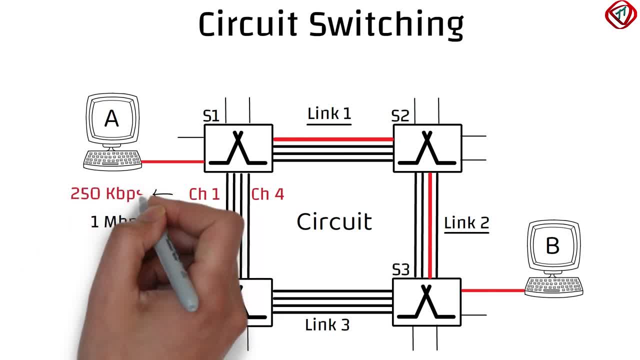 channel has a transmission rate of 250 Kbps. Hence each end-to-end connection gets a dedicated transmission rate of 250 Kbps. Such a network, where sender-to-receiver connection receives a guaranteed constant transmission rate with the help of reserved resources, is called a circuit. 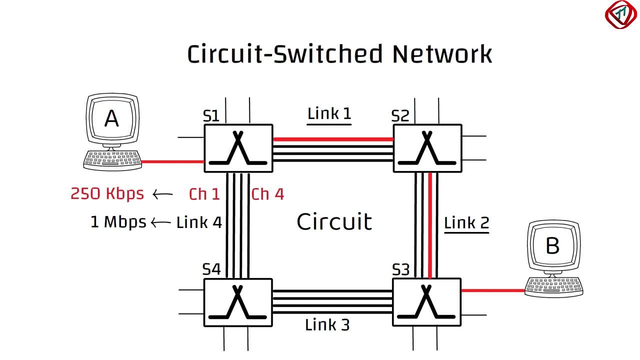 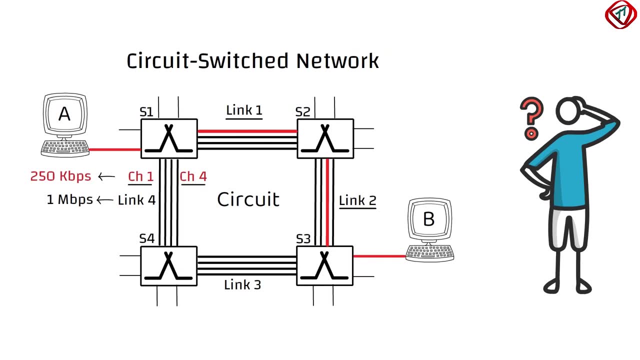 switch network And the switches are called circuit switches. In the current network, each link has 4 channels. These channels, or the combination of channels, are reserved for one-to-one communication. So what exactly these channels are and how they are established. 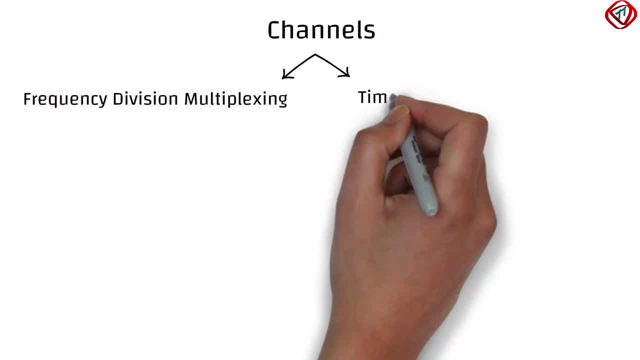 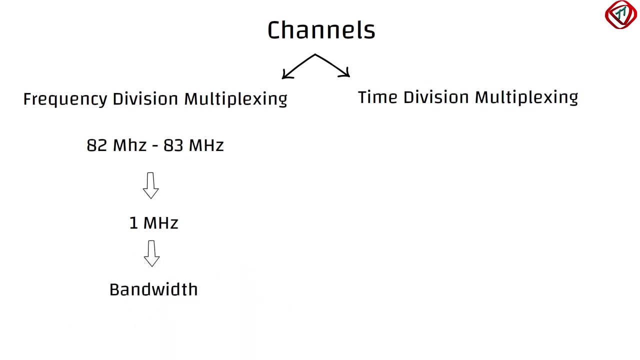 The channels are created with frequency division multiplexing or time division multiplexing. Suppose you have a frequency range of 82 MHz to 83 MHz. The difference between higher and lower frequency is 1 MHz. It is called bandwidth. The channels are bandwidth in frequency division multiplexing and time slots in time division. 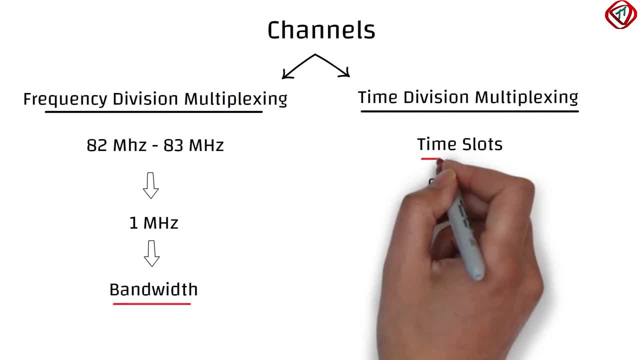 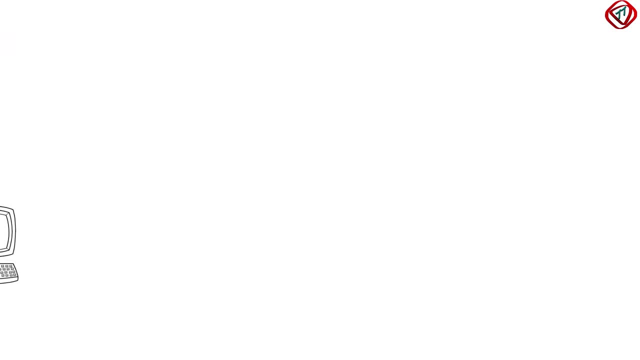 multiplexing. So bandwidth or time slots are reserved for sender-receiver pairs in a circuit switch network. Communication in a circuit switch network involves three phases: Connection setup phase, data transfer phase and connection tiered phase. So the channel is called a circuit. 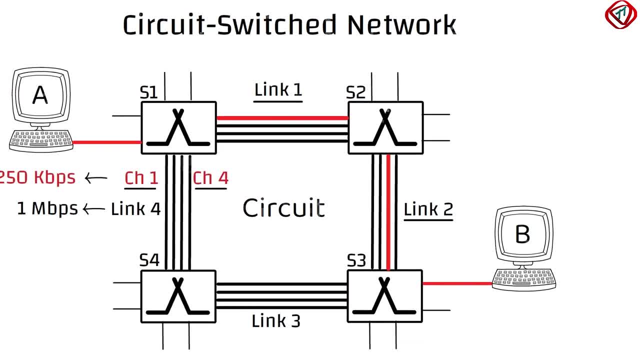 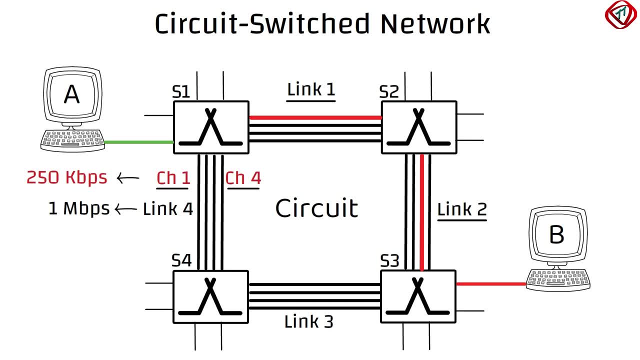 's connection tier-down phase. Suppose host A needs to setup a connection with host B. Host A sends a connection setup request to switch 1.. This request contains the address of host B. Switch 1 finds a channel between itself and switch 2 that can be reserved for the. 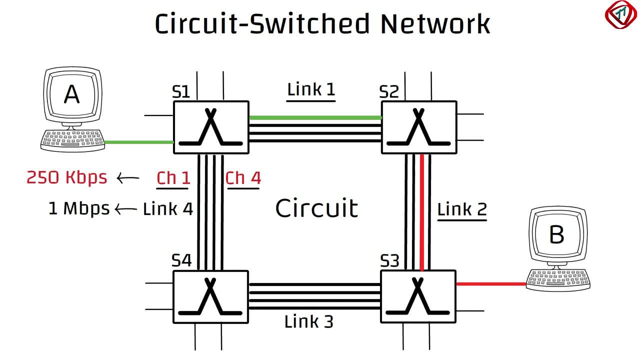 communication session. Switch 1 then sends the request to switch 2.. Switch 2 finds a channel between itself and switch 3.. Switch 2 finds a channel between itself and switch 3.. Switch 2 then Switch 3 then informs the host about the connection request. 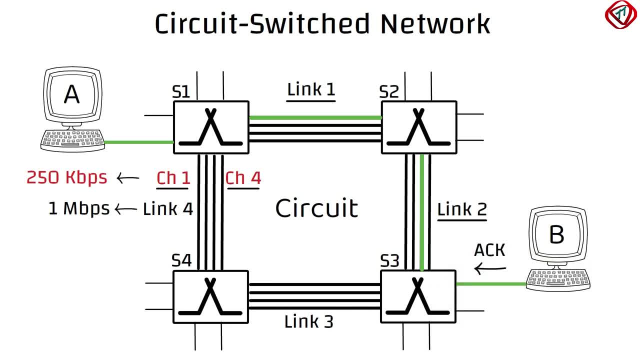 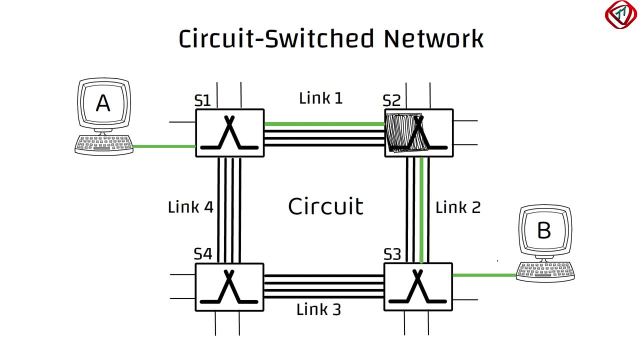 Host B accepts the request and sends an acknowledgement message to host A. Once host A receives the acknowledgement message, the circuit is established. It is called connection setup phase. After the circuit is established, host A and host B can transfer data. It is called the data transfer phase. 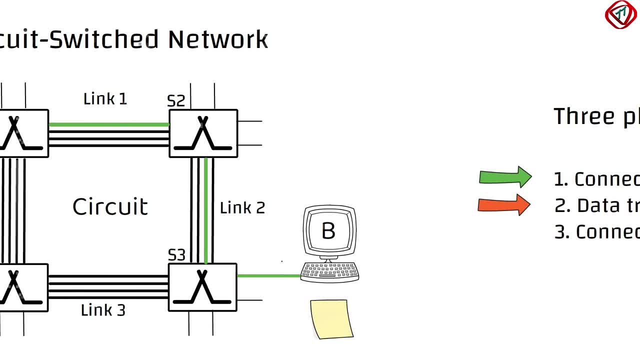 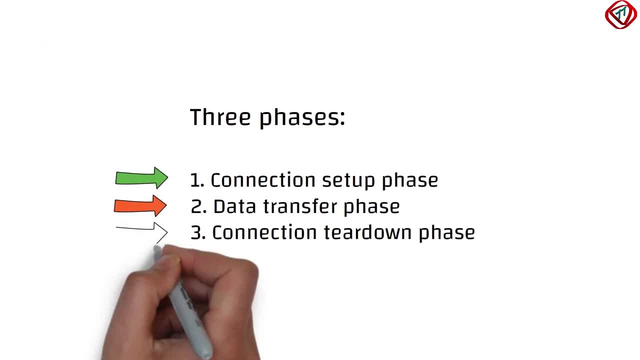 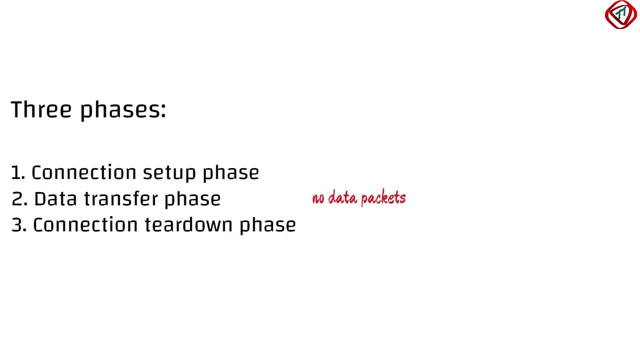 When one of the two hosts need to disconnect, a signal is sent to the switches to release the resolved resources or channels. It is called the connection teardown phase. Please note that the data in circuit switch networks is not in the form of packets and no addressing is involved during the data transfer phase. 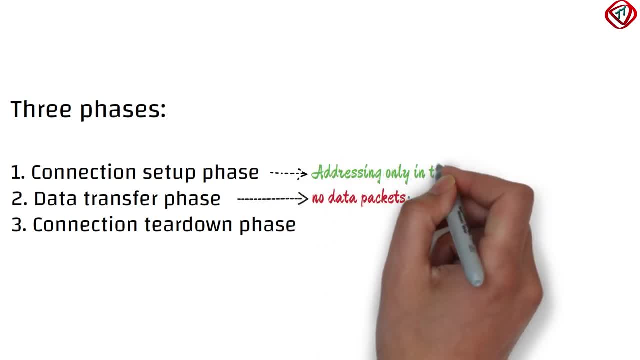 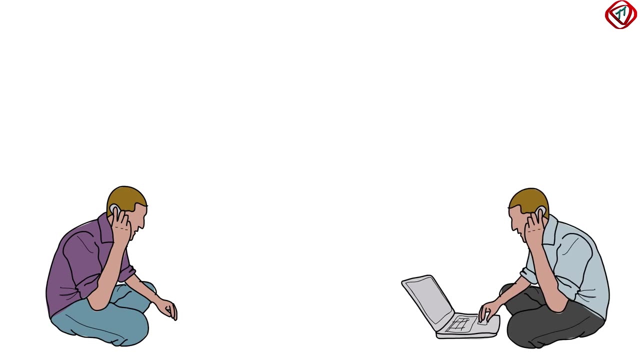 Addressing is used only in the connection setup. request to reserve channels for one-to-one communication. After that, the data from sender to receiver is a continuous flow Circuit. switching takes place at the physical layer. Suppose a person is talking to his friend. 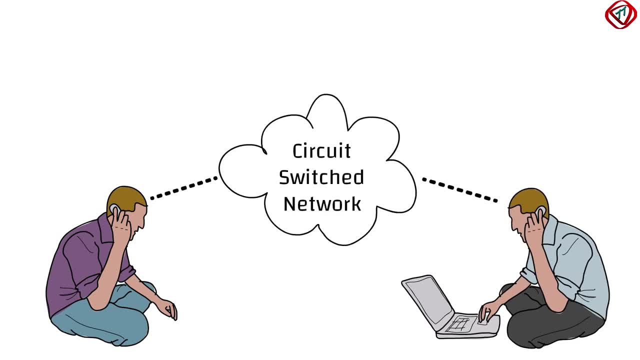 After some time, both of them stop talking for 5 minutes. For these 5 minutes, the reserved resources are idle and cannot be used by any other ongoing communication because they are reserved for their communication session only. Due to this reason, the circuit switch networks are not available. 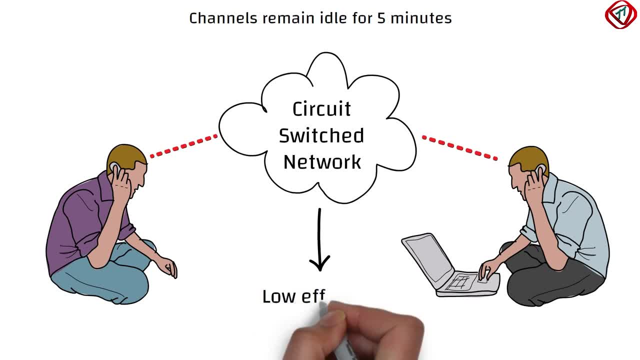 This is the reason why the circuit switch networks are not available. After that, the data from sender to receiver is a continuous flow. The circuit switch networks have low efficiency. However, the delay in this type of network is minimal because there is no waiting at.